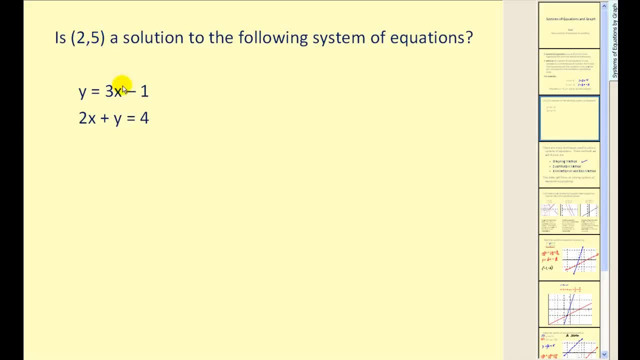 we have to make sure, when x equals 2 and y equals 5, that it satisfies both equations, not just one. So if we take a look at the first equation, we'll replace y with five and x with two and see if it's true. 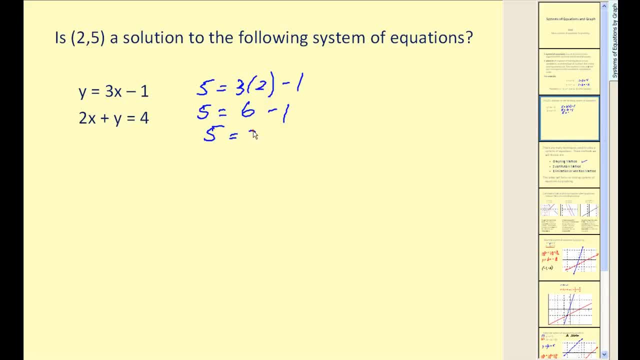 We would have five equals six minus one, or five equals five, which is true. Now we must do the same to the second equation. So we'd have two times x, which is two, plus our y value, which is five, is equal to four. 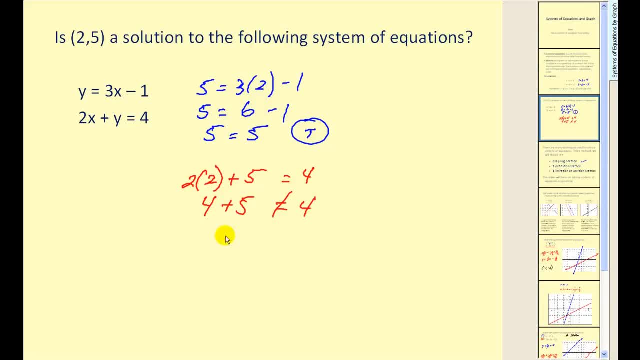 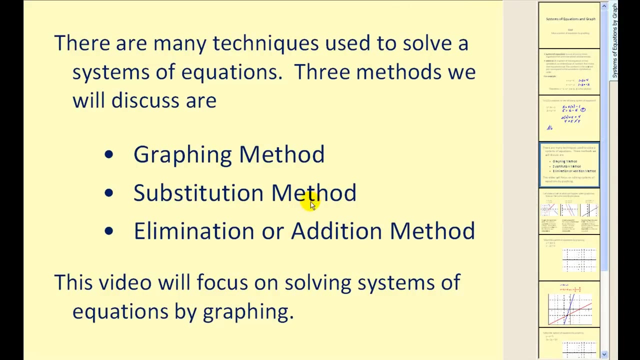 So four plus five is equal to four. Well, that's not true. Therefore, two five is not a solution to this system. Now, this video focuses on solving a system of equations by graphing. There are two other methods we'll look at in future videos. 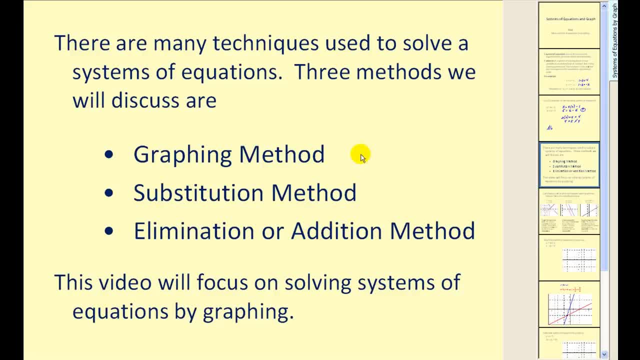 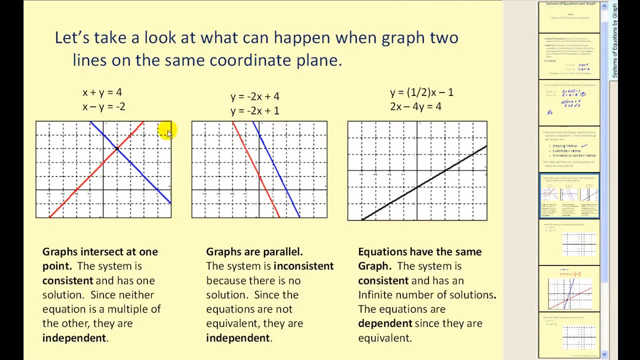 called the substitution method and the elimination or addition method, But again, today we'll only be focusing on the graphing method. So what we're going to do is graph each equation on the same coordinate plane and then analyze the results. All of our equations will be linear. 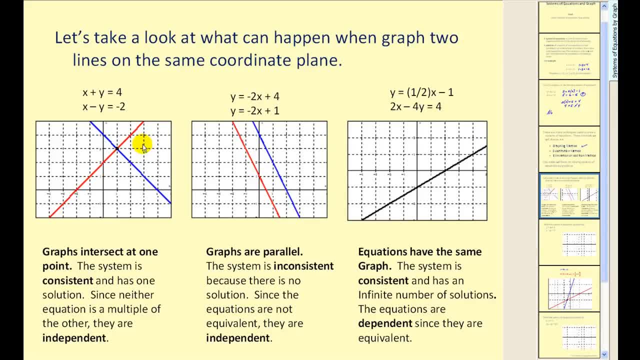 so three things can happen when you graph two linear equations on the same coordinate plane. The first possibility is you have one point of intersection, and this point of intersection here would be the solution. So if this was our system, the solution would be x equals one and y equals three. 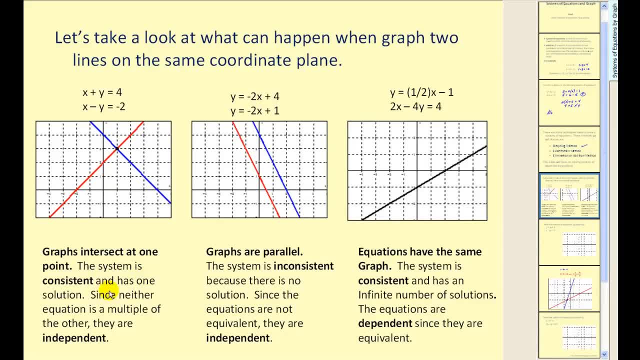 If the graph intersects at one point, the system is considered consistent and also independent. Another possibility is we could have two lines that are parallel to each other, And on this case the lines don't share any points. therefore there is no solution. 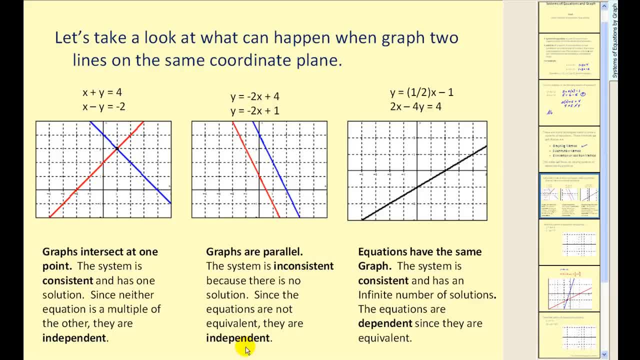 and the system is called inconsistent and independent. But the main idea here is: there's no solution. Third case is: if we graph both lines and they happen to be the exact same line, then we have an infinite number of lines. So if we graph both lines and they happen to be the exact same line, 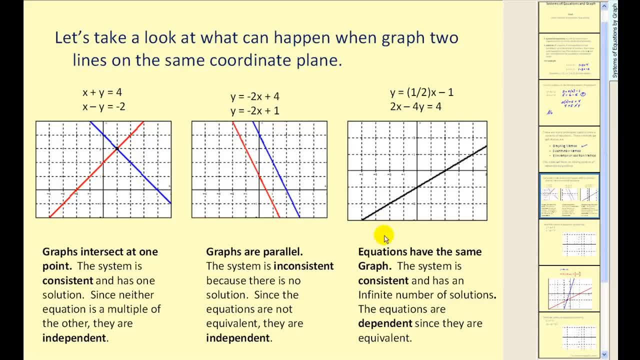 then we have an infinite number of lines. Then we have an infinite number of lines. So if we graph both lines and they happen to be the exact same line, then we have an infinite number of points in common between the two lines. therefore, we have an infinite number of solutions to the system. 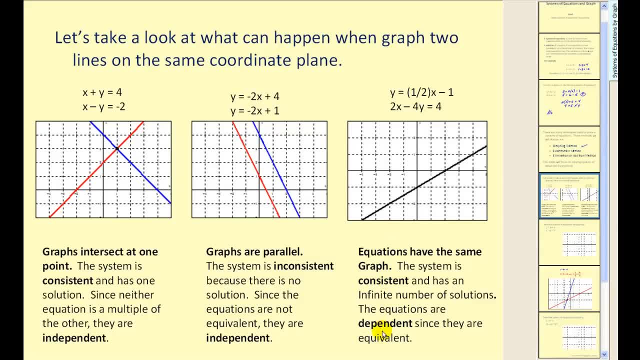 And this type of system is considered consistent and dependent. So, in general, if the system has at least one solution, we call it a consistent system, And if the two equations are different, we have an independent system. And if the two equations are the same, 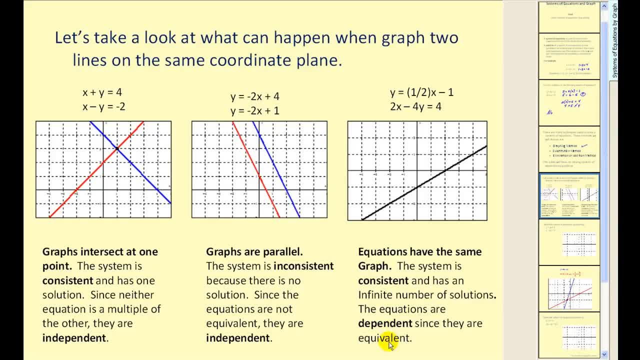 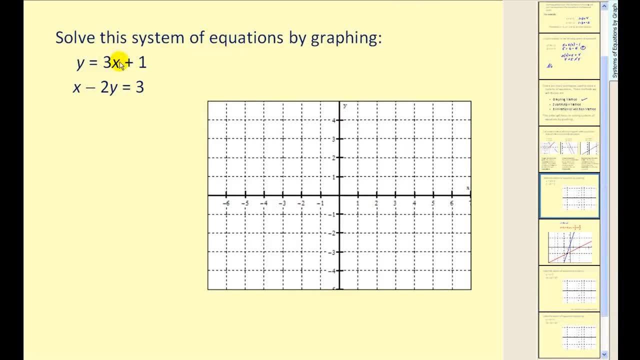 we have a dependent system. I don't focus too much on this vocabulary, but your instructor may. Okay, so let's give it a try. We want to solve this system by graphing, So what we're going to do is graph the first line. 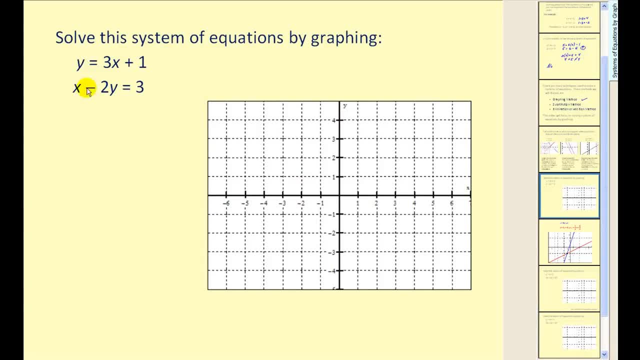 graph the second line and analyze the results. So in order to graph this first line- it's in sloped intercept form- We have a y-intercept of positive one, We have a slope of three or three over one. So from the y-intercept we'll go up three and right one. 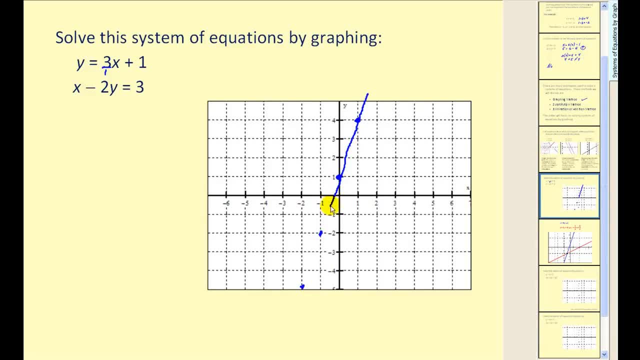 So our line passes through these points. Next, on this equation, it's not in sloped intercept form, so we can make a t-table, we can find the intercepts, But I'm going to go ahead and solve this for y. 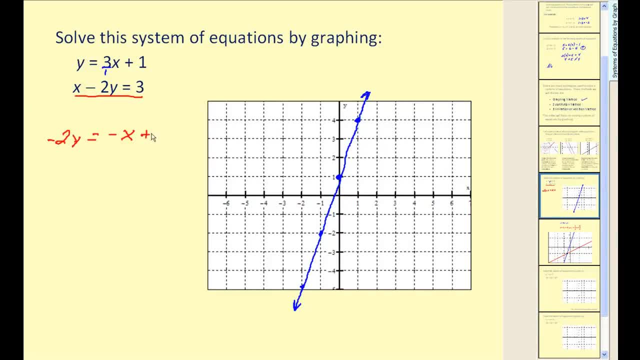 so I'll subtract x on both sides, Then divide by negative two, So we have: y is equal to one-half, x minus three-halves. So our y-intercept is negative three-halves or negative 1.5.. Our slope is one-half. so from here, 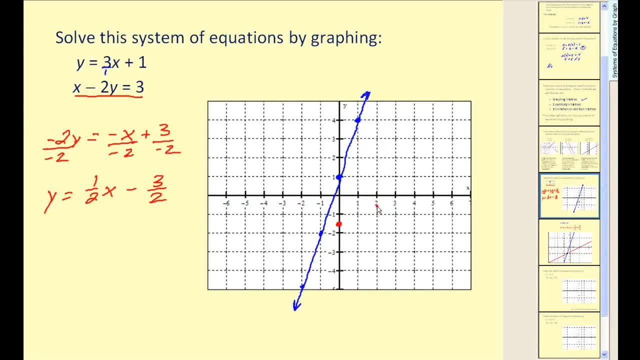 we'll go up one and right two, And I'm going to go ahead and find a few more points. So our second line passes through these points. We can see that there is a point of intersection. therefore, we do have one solution. The coordinates of that point represent our solution. 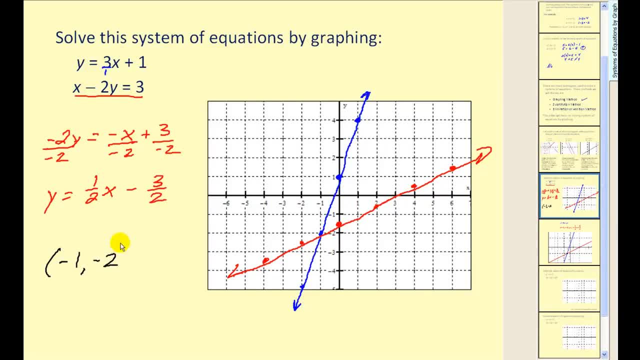 of negative one, negative two. So x is negative one and y is negative two. Now you can see right away. one of the disadvantages of graphing to find a solution is you have to be extremely accurate and sometimes that's very difficult. 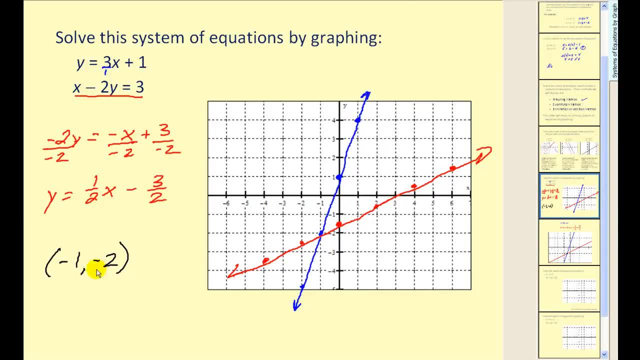 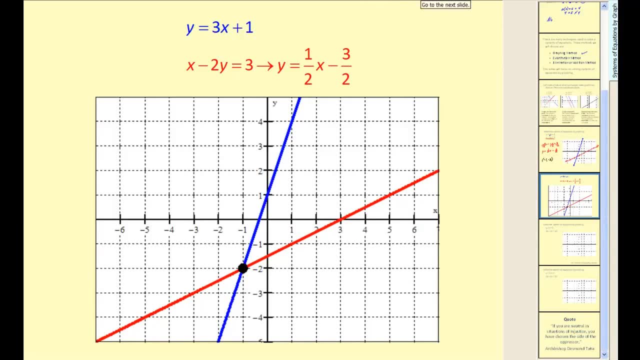 especially if the x and the y coordinates are not integers. Here's another look at it using a graphing program. We'll take a look at how you can do this on your graphing calculator. on the next problem, So again, we'll graph these two lines. 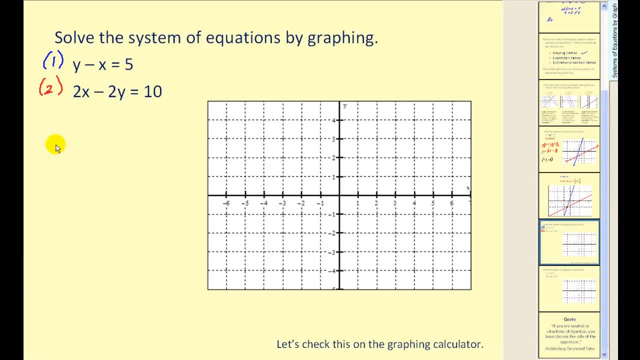 and then analyze the results. So for the first line, if we add x to both sides, we'd have y equals x plus five. so we have a y-intercept of positive five and a slope of positive one or one over one. 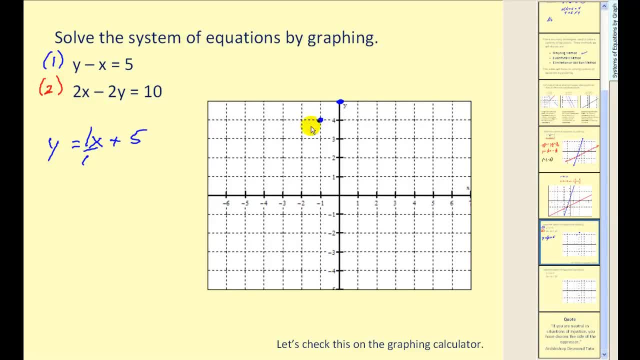 Since I can't go up one and right one, I'll go down one and back one. The result would be the same, and so our line passes through these points. On the second line, I'll first start by subtracting two x on both sides divide by negative two. 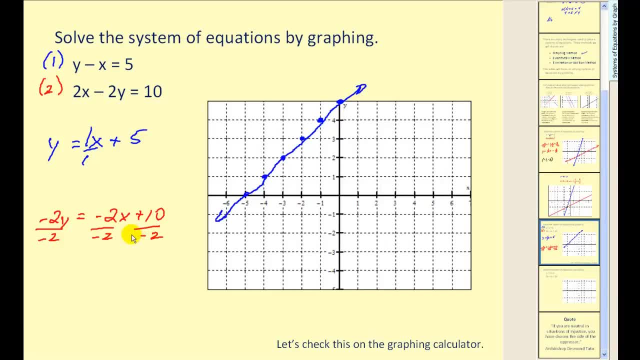 to obtain y equals x minus five. So here we have a y-intercept of negative five and a slope of positive one. So again, we'll go up one right one several times to get additional points. So our second line would look like this: 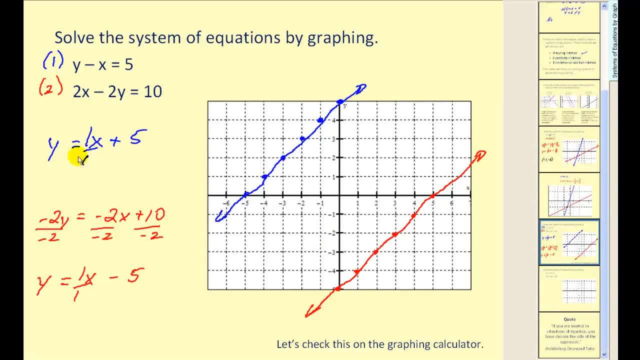 And what we see here is these two lines are parallel, and that does make sense, because our slopes are both equal to one and our y-intercepts are different. Therefore, this system has no solution, which we could also classify as inconsistent. 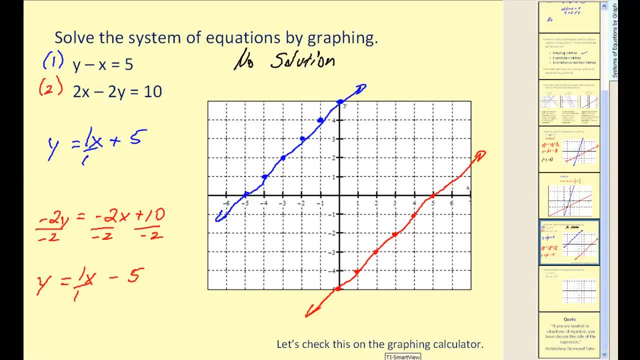 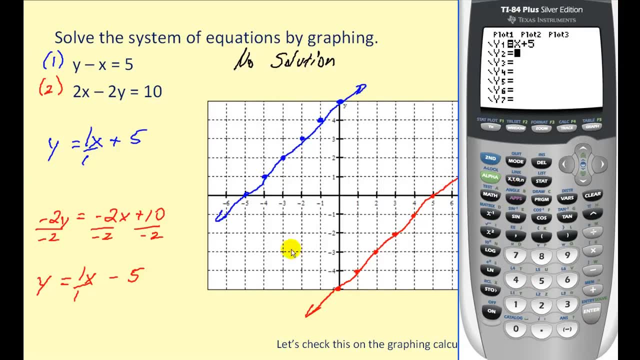 and independent. Now let's take a look at our graphing calculators just to verify this. What you can do is type first equation in y, one which is x plus five. Type in the second equation into y two x minus five. 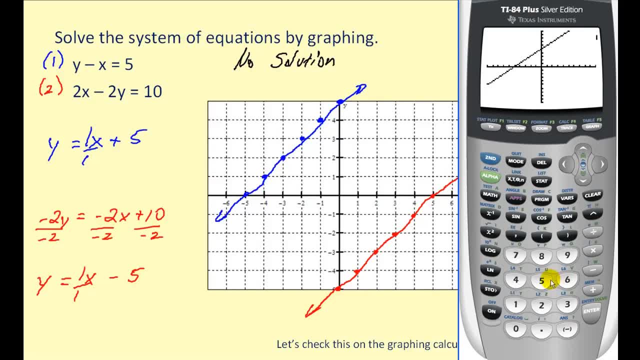 We'll hit zoom six to get the standard window. And again, this verifies our work. Now, if there is a point of intersection, the way you can find it is if you hit second trace and then option five for intersection, and then if you hit enter three times. 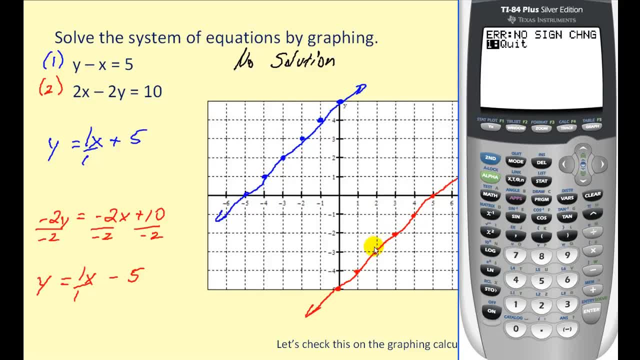 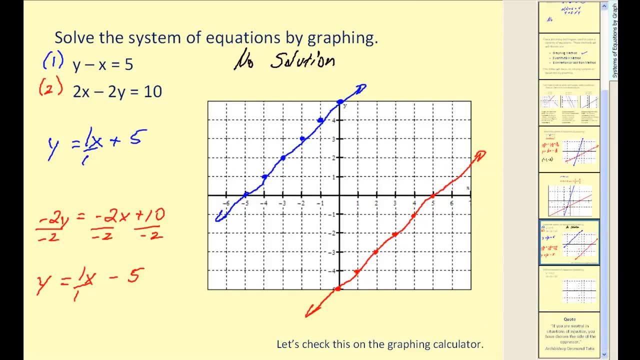 Now we got an error because there was no point of intersection, but if there was, it would tell us the coordinates of the point of intersection. So, for example, if I went back to the first problem that we did and just to double check this, 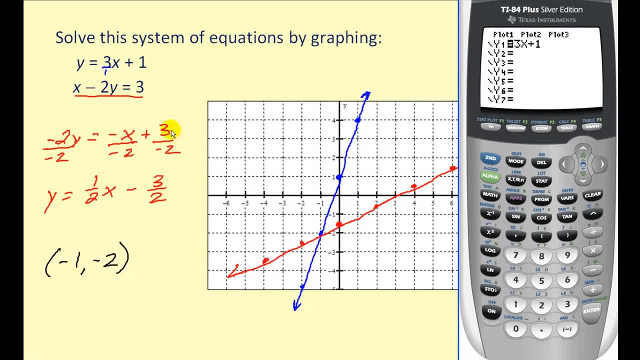 if I type the first equation in y one, the second equation in slope-intercept form into y two, we do have to wrap up our slope in a set of parentheses and hit. graph Matches our graph perfectly and just to verify if we hit second trace.